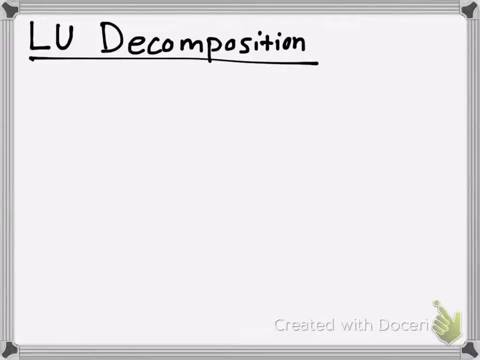 do two examples. Alright, so LU decomposition in terms of how you do it, we'll start with that. Two main steps. one row reducer matrix is normal. like many steps you do in linear algebra, you always start with row reduction. Second step you're going to want to do is 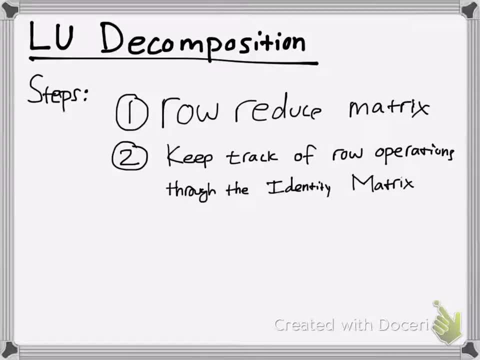 keep track of your row operations through the identity matrix. So if you know of elementary matrices, it's kind of showing the action done onto the matrix and you keep track of those using the identity matrix. And why is this LU decomposition? what is it exactly? 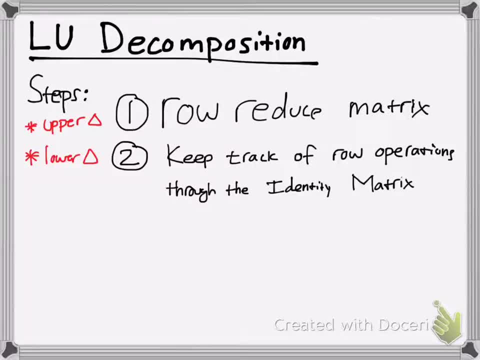 Well, you're splitting up a matrix into an upper triangular matrix and a lower triangular matrix. So A is your matrix and you have your upper or lower triangular and your upper triangular matrix And you're thinking like, what's the point of splitting? Well, you're. 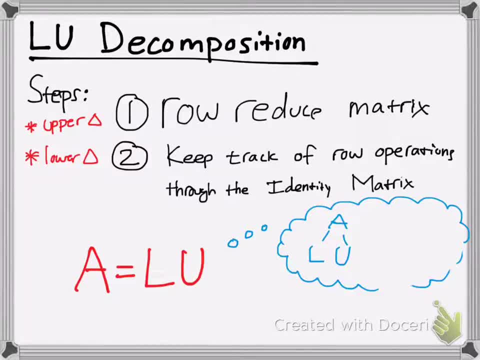 splitting it up. well, it's kind of how I like to think about it. It's A factors to LU. it's kind of like saying 15 is like 5 times 3.. It's just another way of showing what the number 15 is. it can be written as 5 and 3, 5 times 3,, excuse me, Just like matrix. 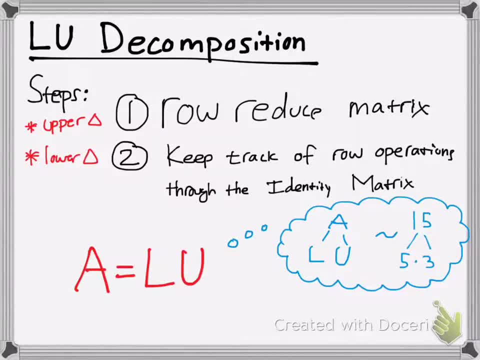 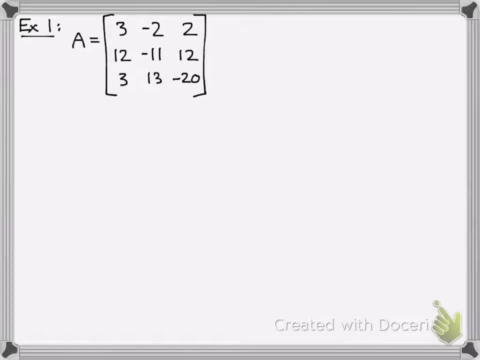 A can be written as L times U. Okay, so that's the concept, that's the steps. let's get into some examples. So you have this matrix A. it's the 3 by 3 matrix. So simple stuff, you're. 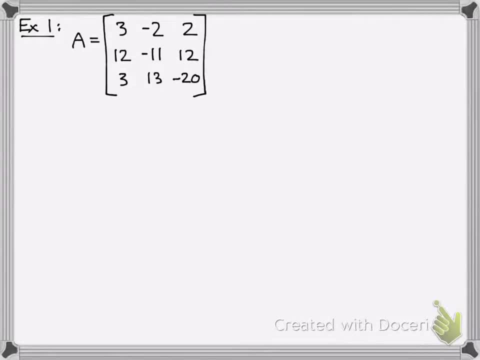 going to want to do row reduction. So you take the pivot, which is the number of rows, use the 3 at the top and you're going to want to subtract 4 from row. subtract 4 times row 1 to row 2.. I'm sure you all know how to do row reduction by now, so I encourage. 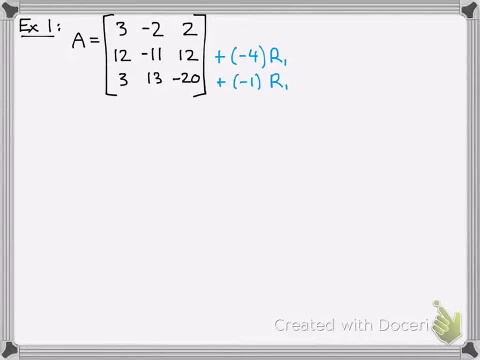 you to pause the video and see what the next steps are. And then you would also subtract row 1 from row 3 in order to get everything below the pivot to be 0. So you should get this as you go across again: So negative 4 times row 2.. 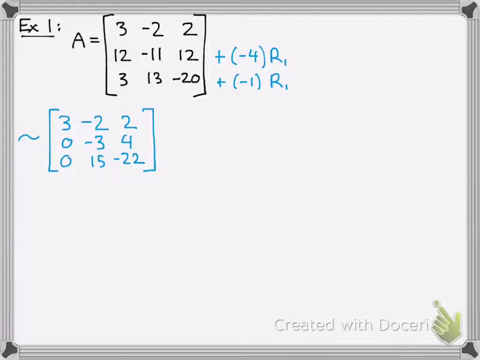 Negative 4 times. row 2 is positive 8, minus 11. is negative 3, negative 4 times. 2 is negative 8, plus 4.. Okay, you get the point. So row reduction, Do it again. you want to make sure. 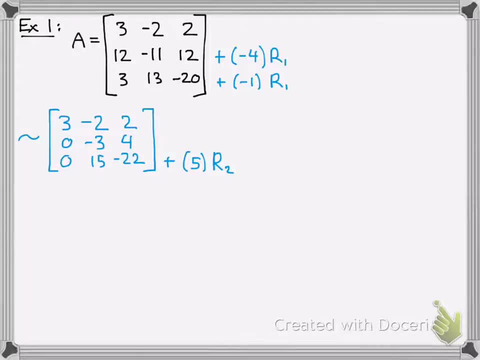 that every pivot has 0 below it, because you're getting an upper triangular matrix. This should be self-explanatory. I'm just going to kind of go through it from now on. So you have your upper triangular matrix, that's your U. 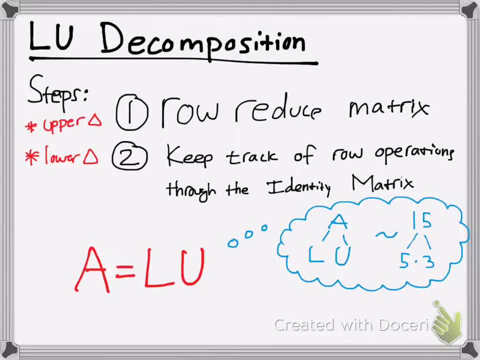 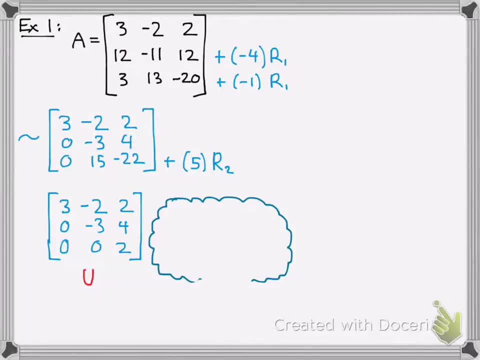 Now, how do you get that Lower triangular matrix? Well, go back to the directions. keep track of row operations through identity matrix. So what were our row operations that we did? Well, let's put them all on a little list here. 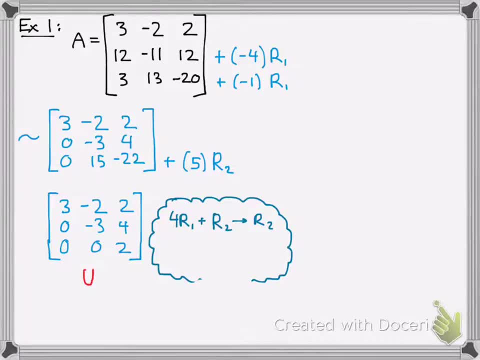 So we did- oops, that should be a negative 4.. Okay Well, we took negative 4 times row 1 plus row 2 to give the new row 2.. Then we subtracted row 1 from row 3 to get the new. 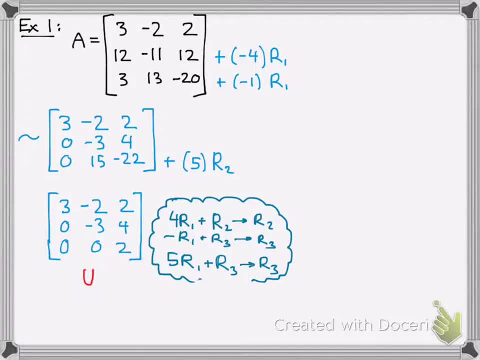 row 3.. And then we have 5 times row 1, excuse me, I should say 2.. So there are a few choices, There are a few typos here. I'll fix those at the end to get the row 3.. I wonder if I 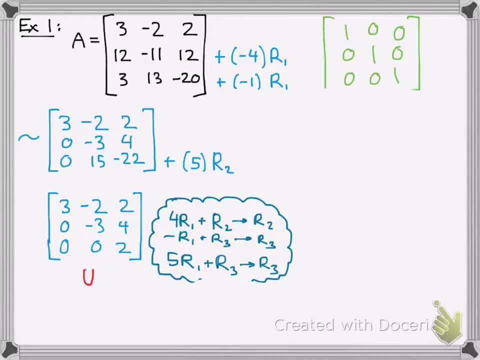 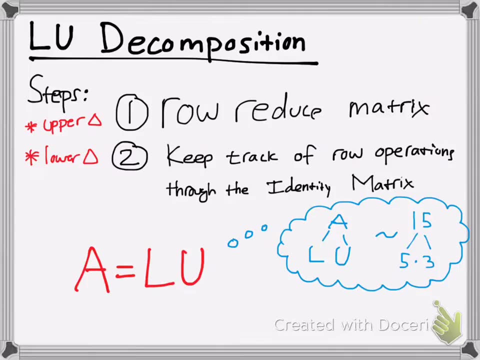 can do that. 2, negative: Nope, I can't, I'm sorry. Okay, Well, get the identity matrix here. So that's part 2, step 2.. Keep track of row operations through identity matrix. So you're going to take these row operations, you're going to do the opposite of them. So 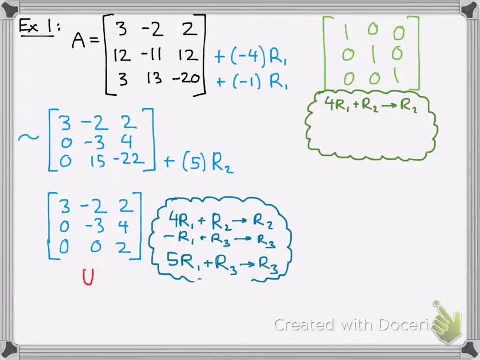 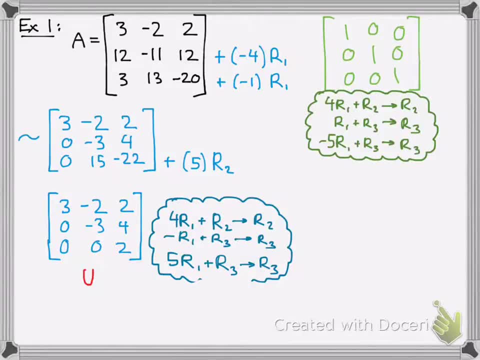 adding 4.. So, instead of subtracting 4, we're adding 4.. So, instead of subtracting row 1 from row 3, we're adding row 1 to row 3.. And instead of adding 5 times row 2 to row 3, we're going. 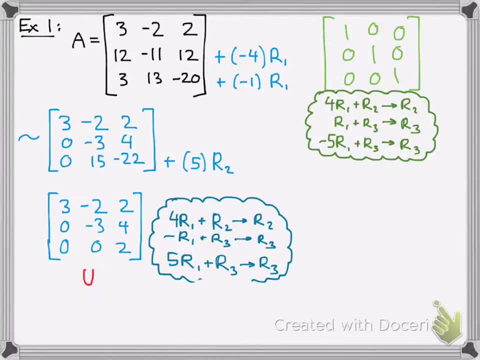 to subtract row 2 from row 3.. That should be a 2 as well. So there are a few typos in here. Please excuse those, But they should be pretty easy to follow. Just take the opposite of the operations that you've done. And now how does that look in the identity matrix? 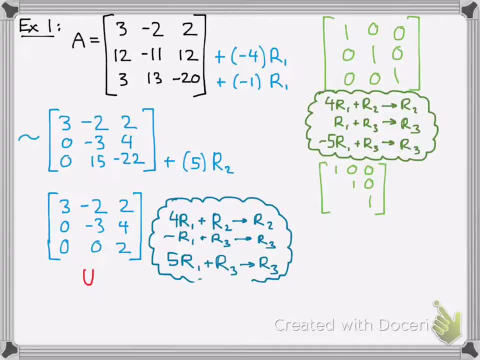 Well, we did 4 times row 1 and row 2.. So where are those numbers going to go? Well, we did the operation on row 2.. So it's going to be in the second row. And what did we do 4 times? 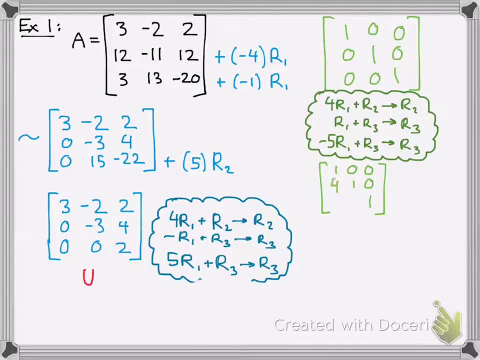 row 1.. So it's going to be in the first column, second row. We're going to put that 4 there. Next, we subtracted. excuse me, we're going to add row 1 to row 3.. So we're doing that. 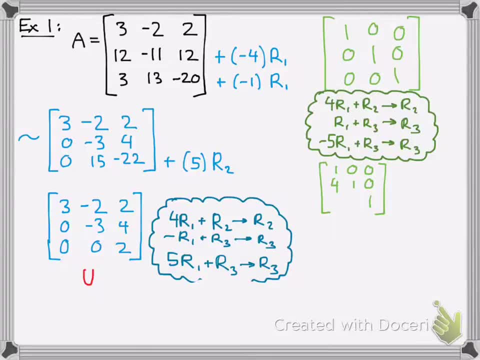 operation on row 3.. So go to the third row of the matrix and we're adding row 1.. So you go to the first column and you put a 1.. Finally you have we are subtracting row 1 from row 3, or 5 times row 1 from row 3.. 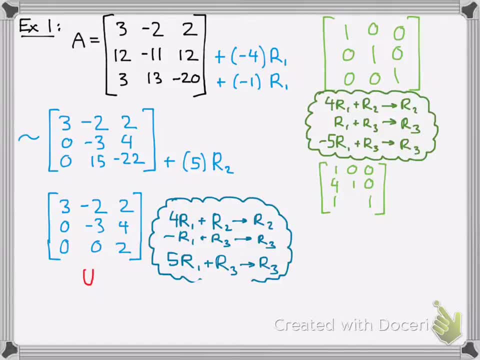 So that is, that should be 2.. That should be row 2.. 5 times row 2. So go again to the third column And then second row, because you're doing the second operation, you get negative 5.. Again, those can be split up into three different elementary matrices to make. 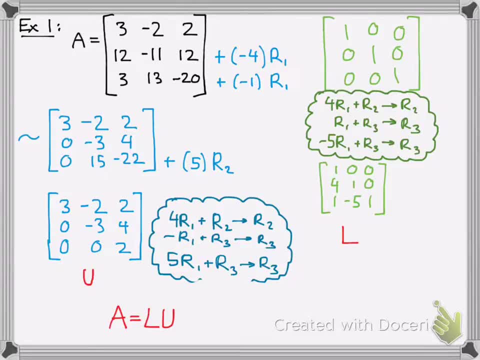 up L, which is the lower triangular matrix. A equals L times U is the formula. It's like splitting it up into its vectors And you simply plug those in that we calculated. So you can check your work by doing matrix multiplication and multiplying these two matrices together. 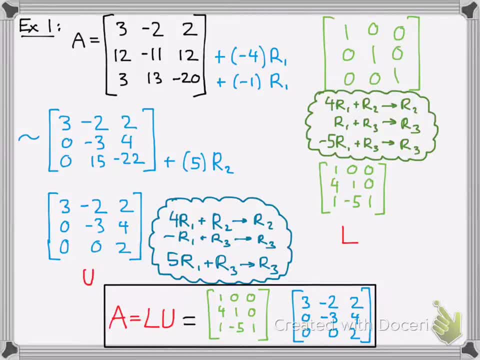 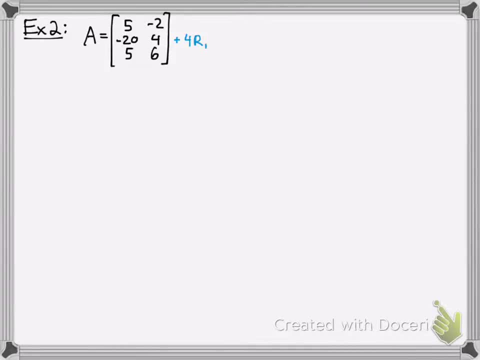 to see if you get the original answer A. This next example will go much quicker, much faster. So here we go. We got our matrix here and we're going to do basic row operations. I pause the video, I suggest, to see what your row reduction looks like. All right, So then? 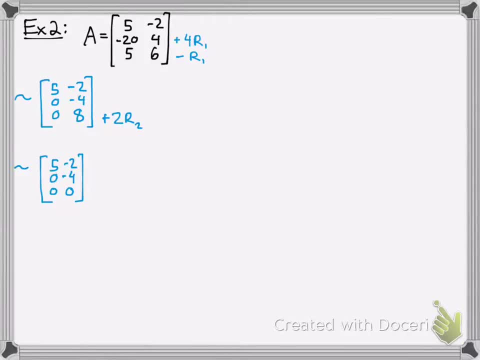 add row 2.. 2 times row 2.. And you should get this when you row reduce. So now that you're here, you have your upper triangular matrix. Now we need to what We've got, to backtrack and keep track of what we did. 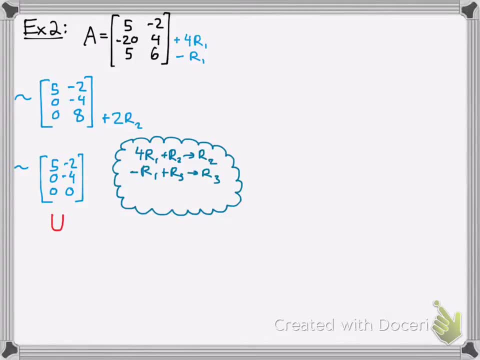 So we did 4 times row 1 to row 2.. We subtracted row 1 from row 3, and we added 2 times row 2 to row 3.. So you're going to want to do the opposites when it comes to the identity matrix. 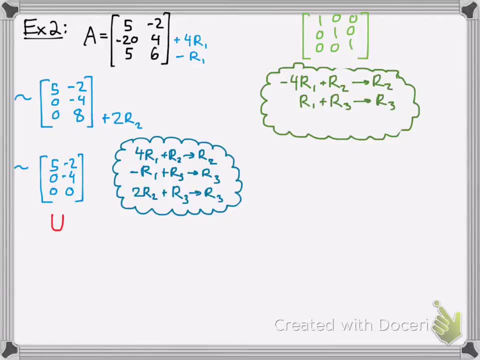 So we're going to subtract 4 times row 1.. You're going to add row 1, and you're going to subtract row 2 times row 2.. Then again plug those into your identity matrix. Same method as last time. 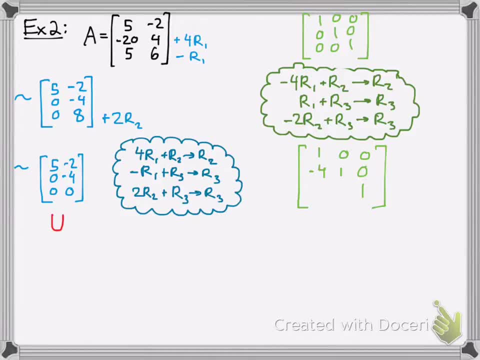 Review your elementary matrices and see how all these numbers show the action that is done onto the matrix. Remember elementary matrices represent the action done onto the matrix. What did you do to manipulate it? Then you have your L and U And remember A is L times U- lower triangular matrix times upper triangular matrix. 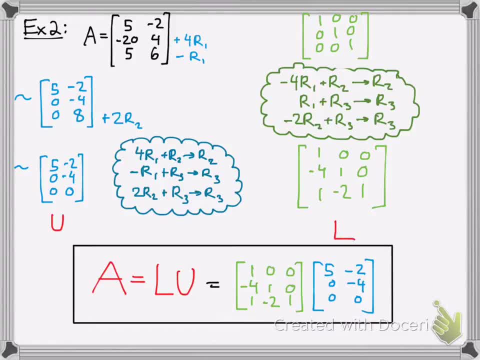 You put them in together and boom, you got it. You're done. This is pretty easy. just a quick example: Pretty much, if you know your row reduction, you know your elementary matrices, you don't have to worry about that.